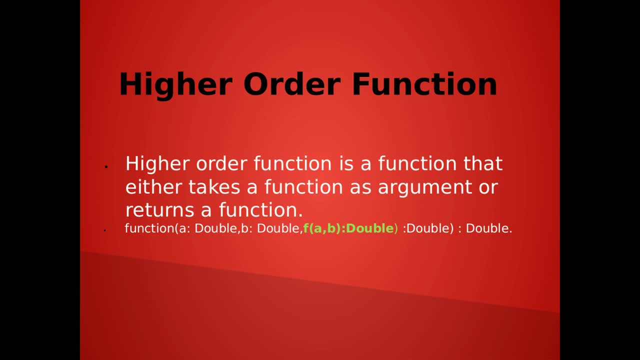 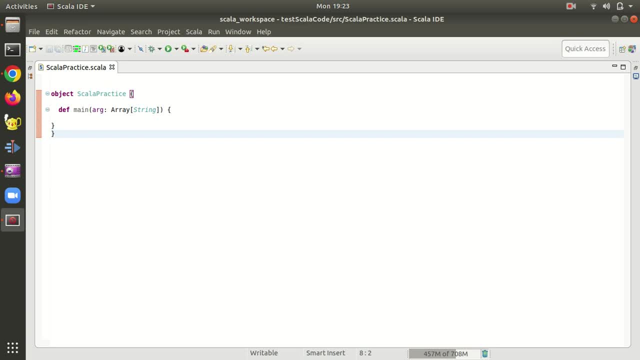 so this is my Scala practice object. so here i'm going to create a function that is a higher order function and and we will use it dynamically. so here i'm creating a function, so my function name is calculate and we are declaring some arguments like, let's say, a: 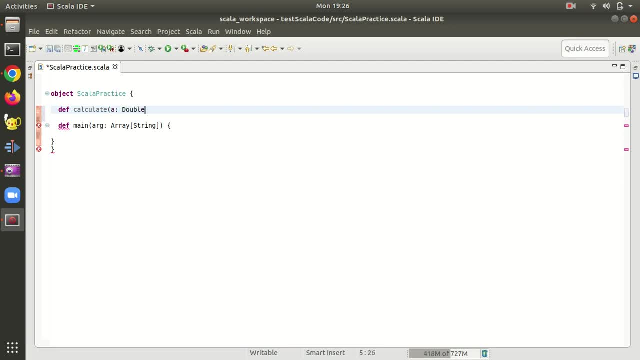 is type of double. similarly, we have another argument, b b, b, and that is also of type double. and then here what we are going to create? we are going to create a higher function that is inside the argument of this function. so suppose the function name is f. 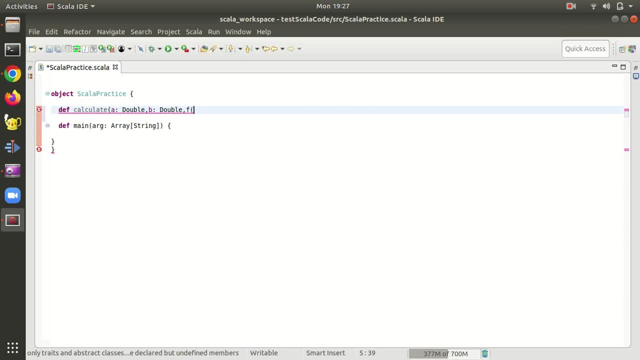 and it will be- must have some arguments. so we are defining its type. its first parameter is double, his second parameter is double, and now we are going to create its body. so what this function exactly do? it takes to double and it returns double. ok, and now we have to create the return type of our calculate. 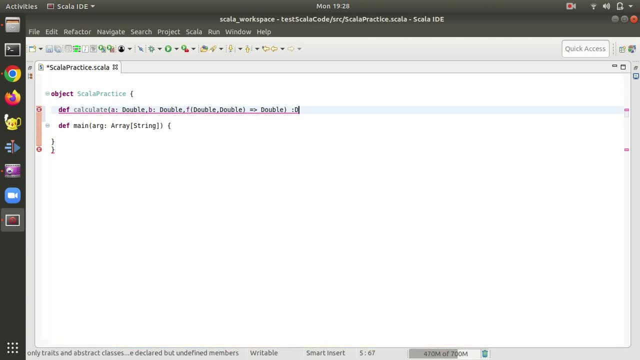 function. so the return type of this calculate function is also double. okay, now this is what the definition. so now we have to create the definition of the function also. that is the declaration of the function, and now we are going to provide the body of our calculate function. so in scalar, how can we do that? you can just write f of f of. 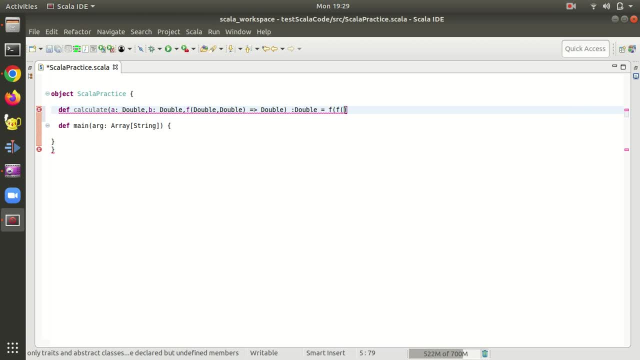 suppose a, comma, b, and so we have to create a body of our calculate function. so how we will create the body of function? so we, we are not doing anything here, we are just returning the value. we are just calling the f function. so we are just calling the f function. 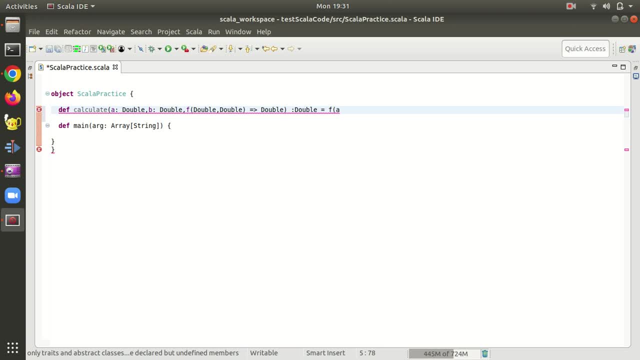 so we are just calling the f function inside our calculate function. so f a inside our calculate function, so f a inside our calculate function. so f a, comma b, comma b, comma b. and okay, so why we are getting this error? okay, okay, so why we are getting this error? okay. 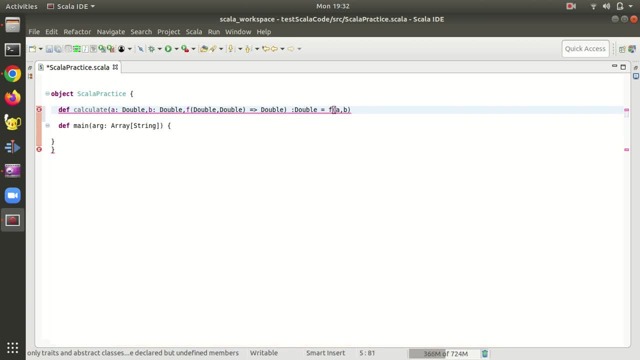 okay, so why we are getting this error? okay, sorry for this? because of this colon, sorry for this because of this colon, sorry for this, because of this colon. one colon is required here. one colon is required here. one colon is required here. so so, so a is a type of double b. 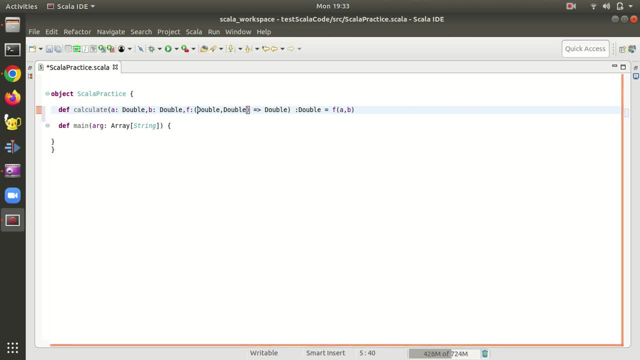 a is a type of double b. a is a type of double. b has double type f. has double type f. has double type f. is a function that contains two arguments. is a function that contains two arguments. is a function that contains two arguments that are double, that are double. 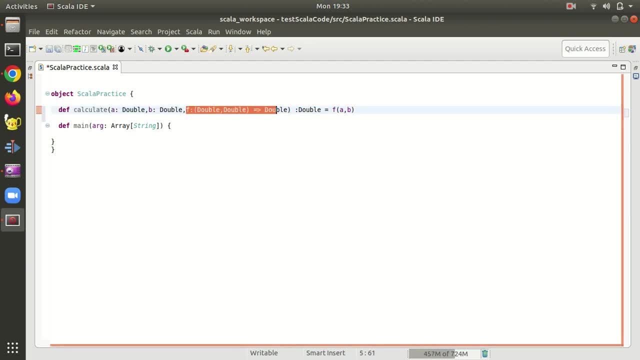 that are double and this f function just written a double value, and for this calculate method we have written type as double to provide the body of this calculate function we are just writing here equals. and from the body of this calculate function we are returning f, that is a comma. 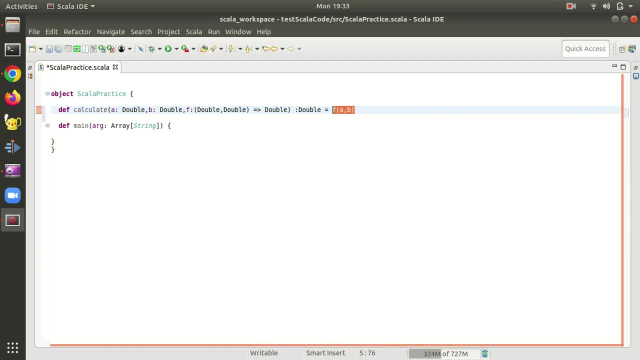 p. if you don't know, I'm not getting what exactly is doing here. I'm just repeating: calculate the function. it's a higher order function that takes one argument as a double. v is a double, f is a function that takes two argument as a double and that returns double. so this: 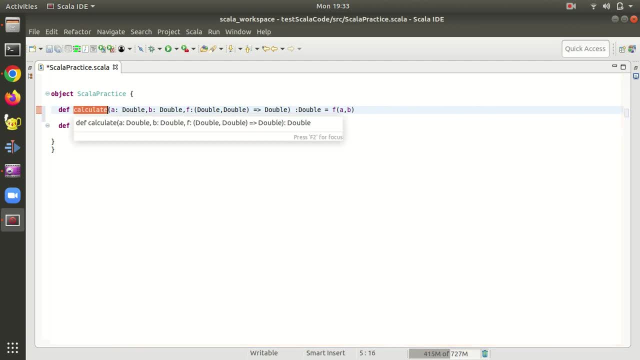 double is a written type of this calculate function and this calculate function inside the body of the function is a comma p calculate function. we are just returning, just calling this function, and when we call this function it will return the value of the return type of this function. So when we call this, 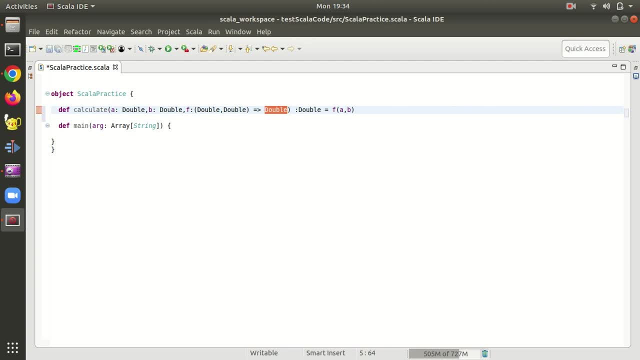 function. it will be clear for us to understand how exactly the function is working. So let's call this function, create a val. result is equals to. we are calling our function. the function name is calculate, So I am passing. the integer is 10. the double value is 10. sorry, 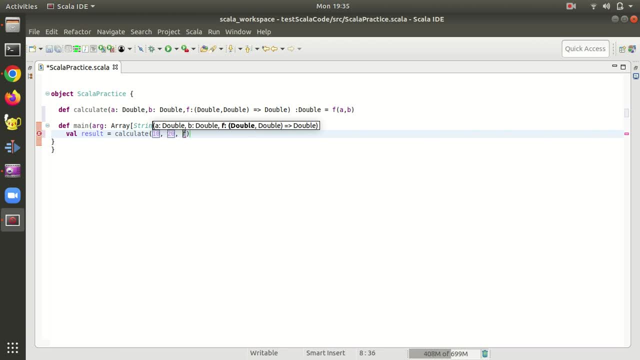 and it is 20.. Now what? what I will pass in the third argument. Third argument is a function which is called function. So I am passing a function which is called argument. So what I have to do here? I will create a function here, just like this. 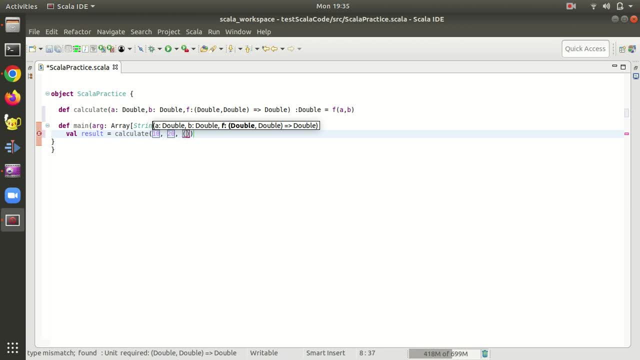 the function that takes two arguments. So the arguments are a comma v and what I am doing with these two values, a comma v. I am just creating a function that can add both the value. So here I am just doing the addition of a and b. So here calculate is a function, and 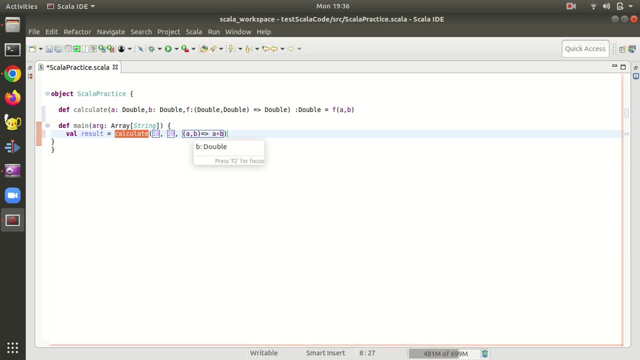 v are the values and whatever I am passing here it is, it will just add both the value. this function and this function will return the result. The result is double, so a plus b result will be here and a plus b result is the last statement of this calculate function. 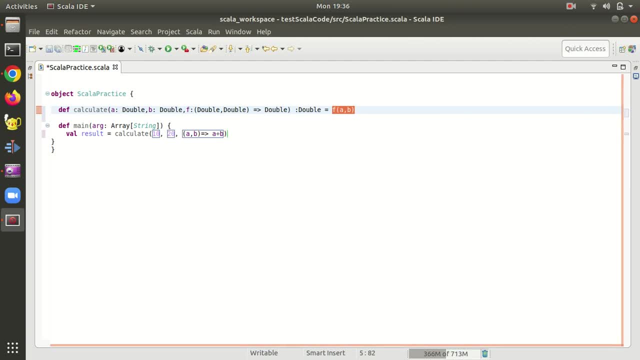 So f a b is the last statement of this function. So whatever f a b will return, the calculate function will return us. So the result will be a plus b, 10 plus 20 is 30. So let's see, Let's print the value of result. 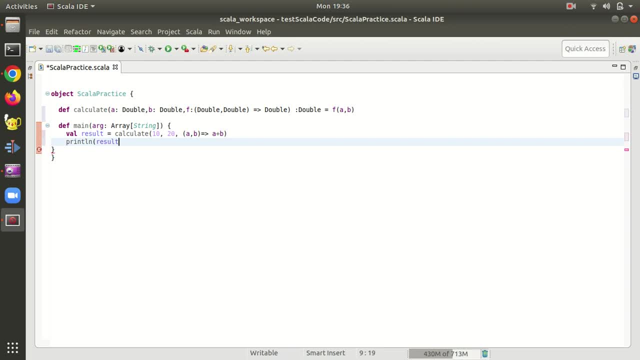 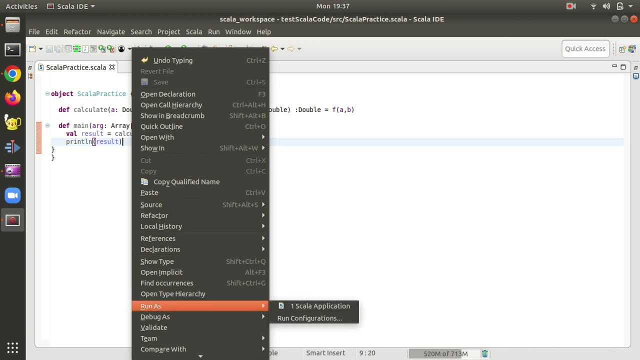 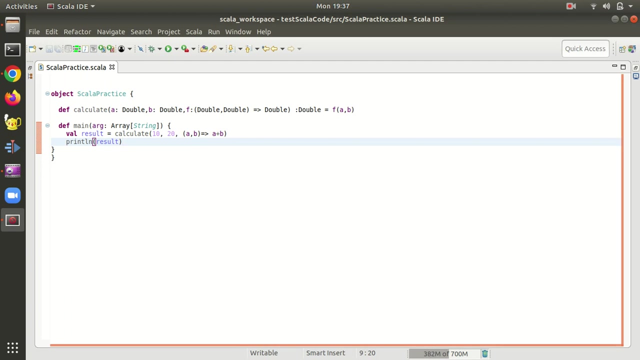 Okay, So our code is complete. So let's run this code run as Scala application. So you can see here in console it is giving me the result 30. So one beauty of the code is I am not writing any logic inside My